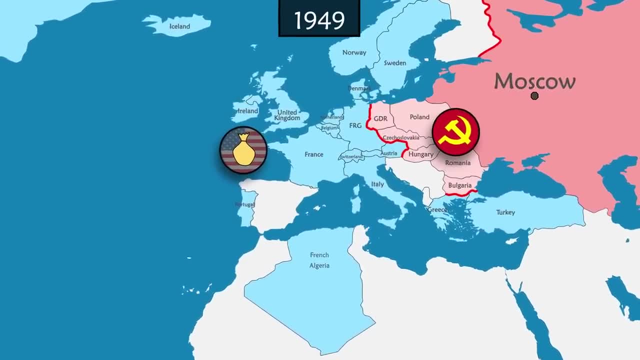 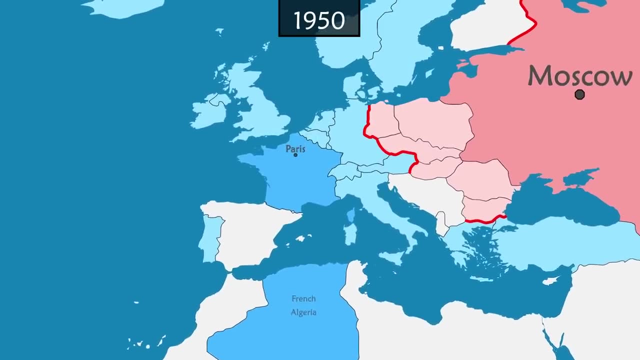 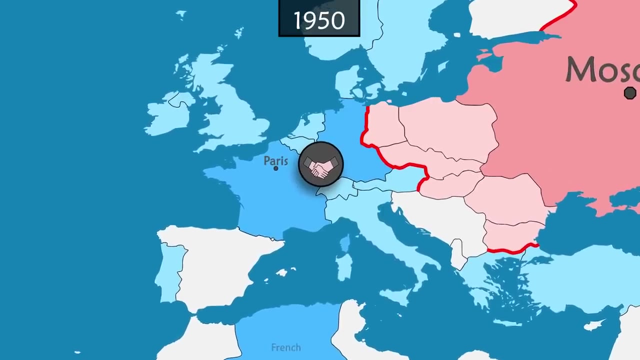 Iron Curtain. in the West, the idea of European Unity begins to take hold. On 9 May 1950, France, via its foreign minister Robert Schuman, proposes a Franco-German reconciliation and placing under a common high authority the production of coal and steel. 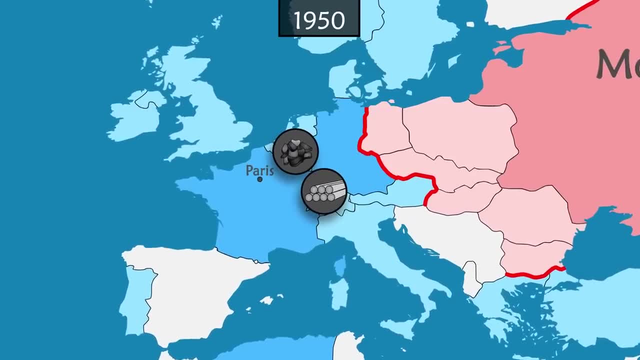 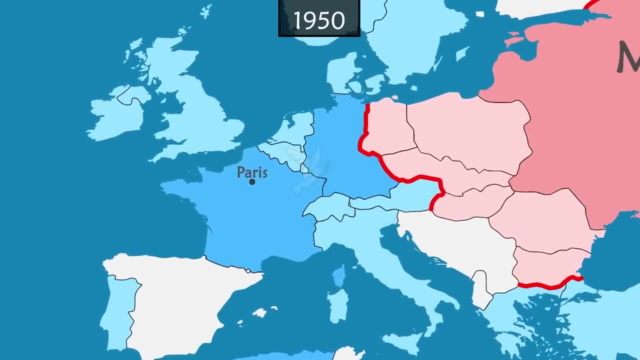 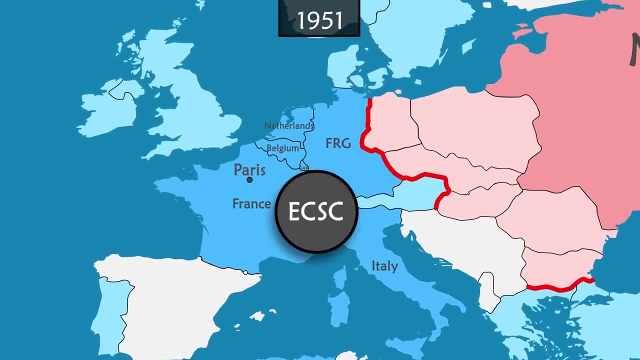 the main wealth of industrialized countries, which is also needed for the manufacture of weapons. The aim is to boost the economy and maintain peace with the project saying project left open to countries wishing to join. The following year, in Paris, six countries sign a treaty establishing the European Coal. 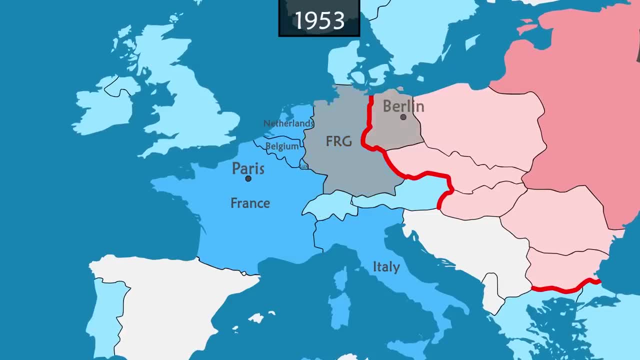 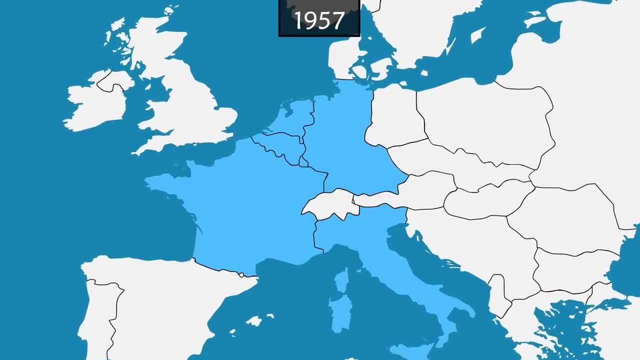 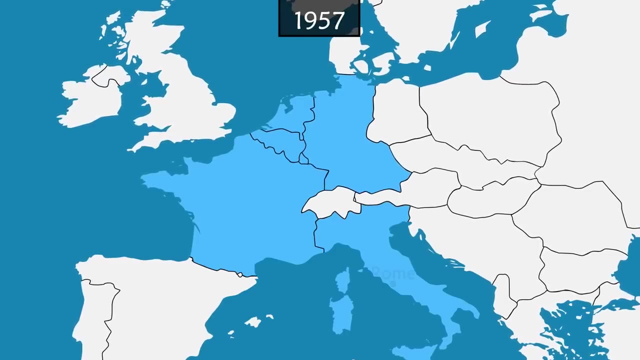 and Steel Community. As Germany is divided by the Iron Curtain, only West Germany becomes part of it. To accelerate the development of Europe, the six founding countries meet on the 25th of March 1957 in Rome to sign two new treaties. 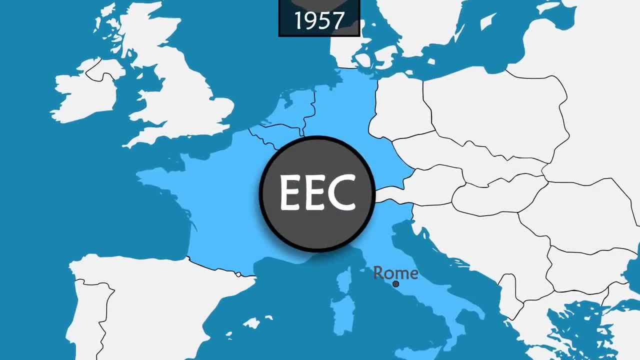 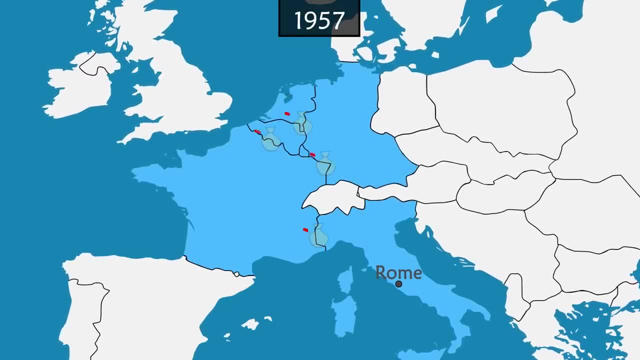 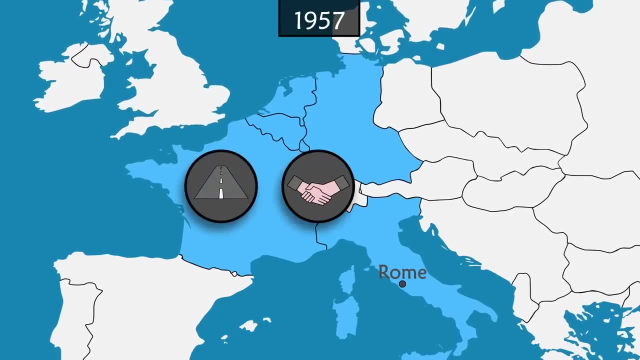 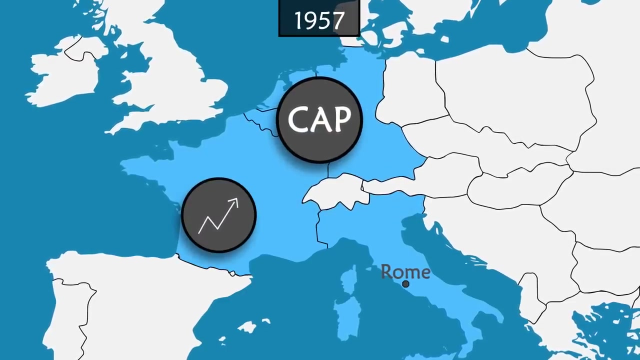 The first treaty creates the European Economic Community, whose main objective is to establish a common market, including allowing the free movement of workers and eliminating tariffs between member states. The treaty also defines common policies on transport, trade and agriculture. The Common Agricultural Policy, among other goals, aims to increase agricultural productivity. 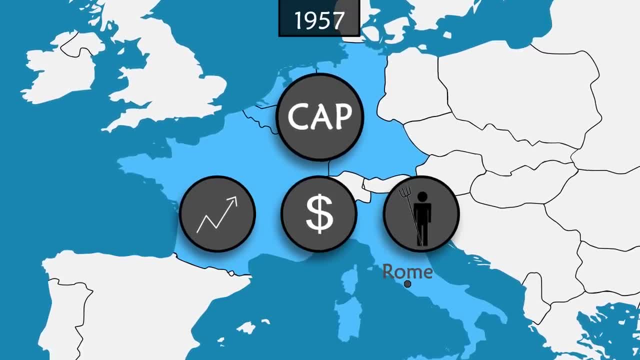 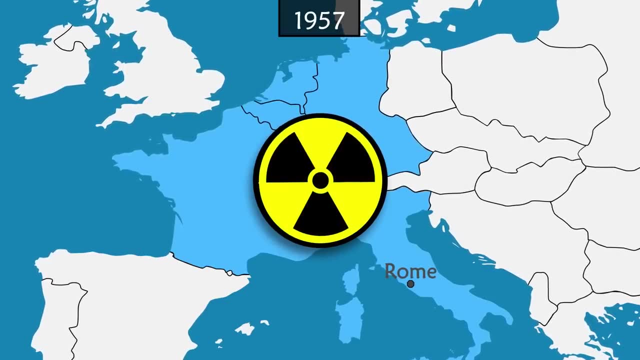 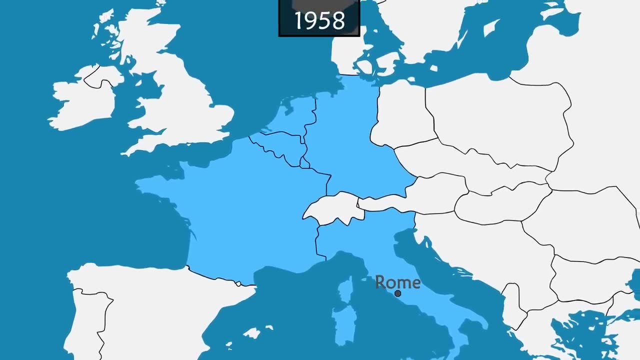 offer reasonable prices and ensure a fair standard of living for farmers. The second treaty establishes the European Atomic Energy Community coordinating civilian nuclear research programs. The treaties of Rome enter into force in 1958, but it would take several years for its policies. 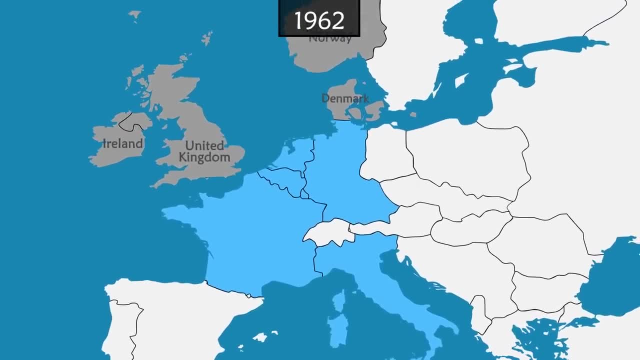 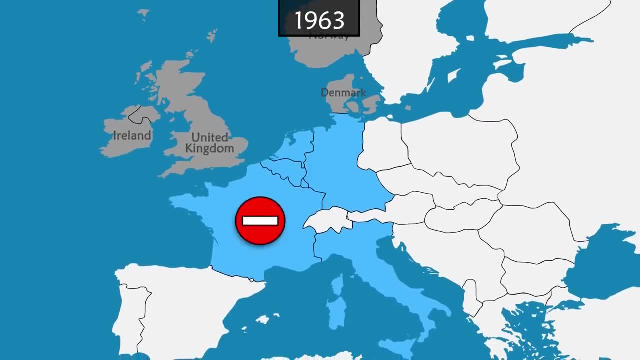 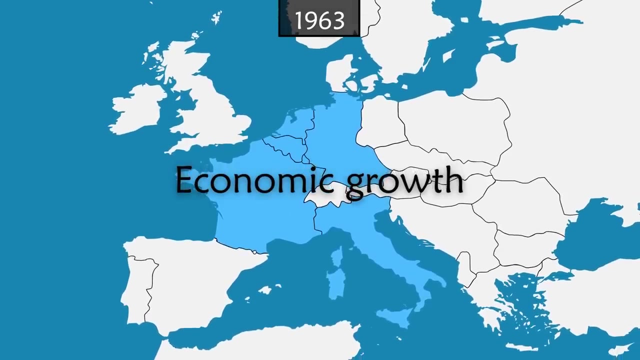 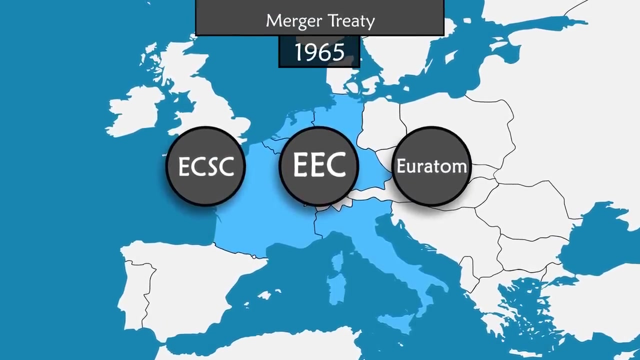 to be implemented. Many countries ask to join the communities, including the United Kingdom, but France, under the leadership of Charles de Gaulle, vetoes the accession request, considering the UK as too close of an ally to the United States. The institutions of the three communities are merged to enable more efficient functioning. 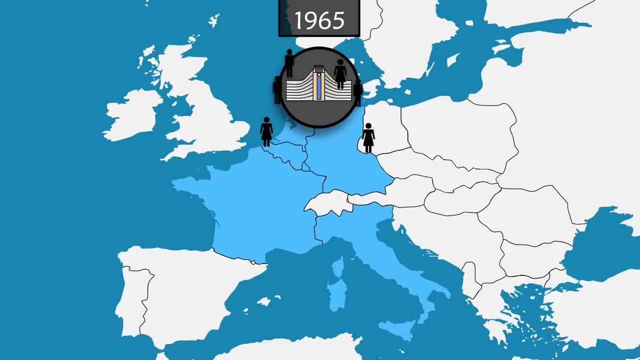 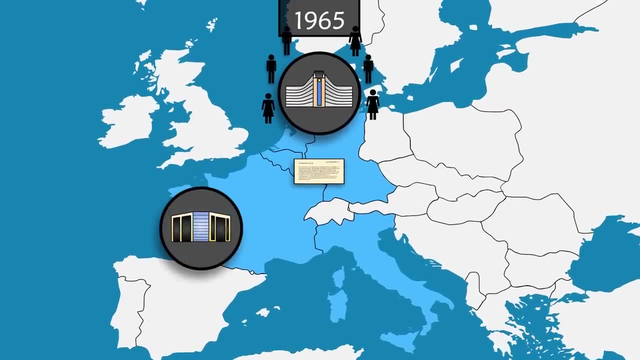 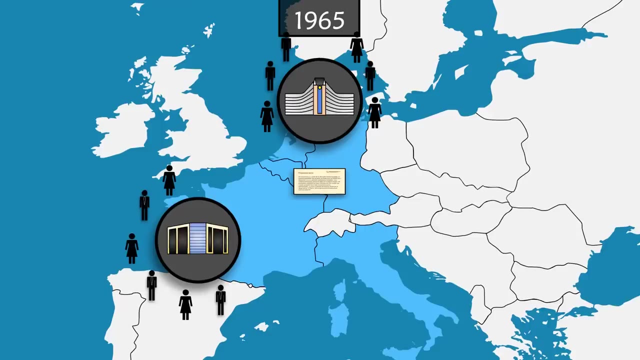 There is now a single commission, composed of commissioners chosen by the heads of state. Its role is to propose European laws in the common interest of its members. There is the council, made up of ministers of the member states and whose role it is to approve, modify or reject the proposals of the commission. 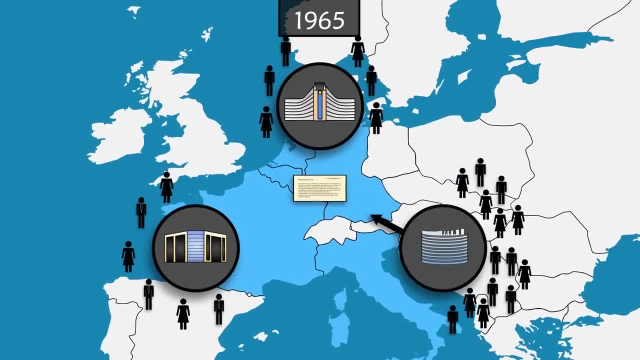 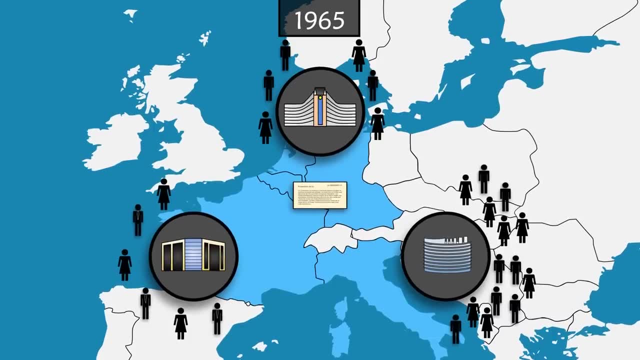 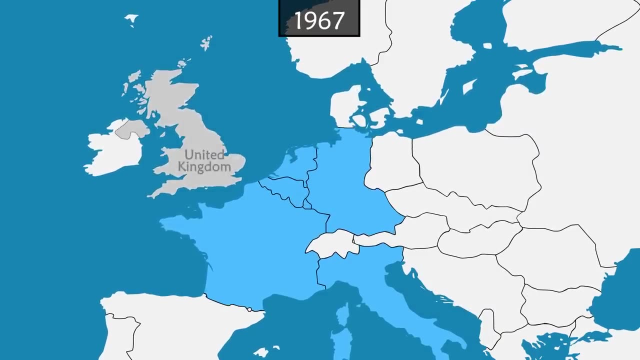 There is the parliament. It represents the people of Europe and which also gives its opinion on commission proposals. Its power would increase over forthcoming treaties. Finally, there is a court of justice that rules over the legality of decisions taken In 1967, the United Kingdom renews its request for membership, which France opposes a second. 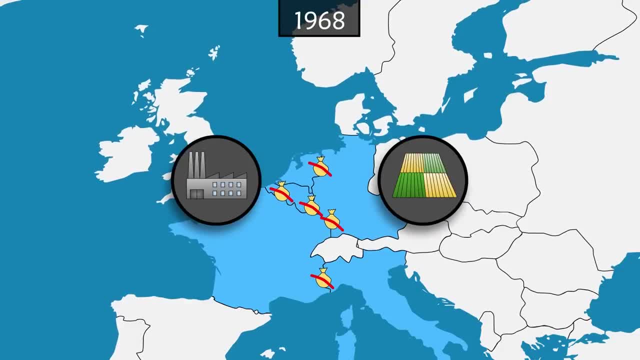 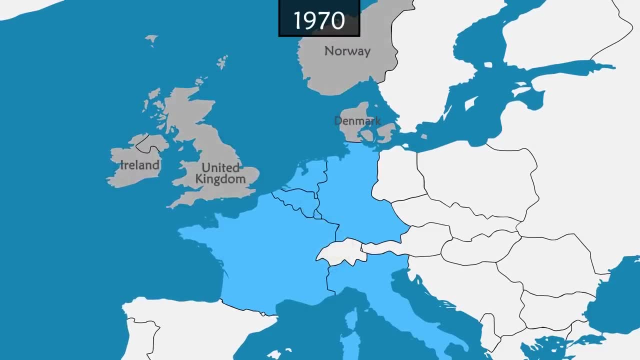 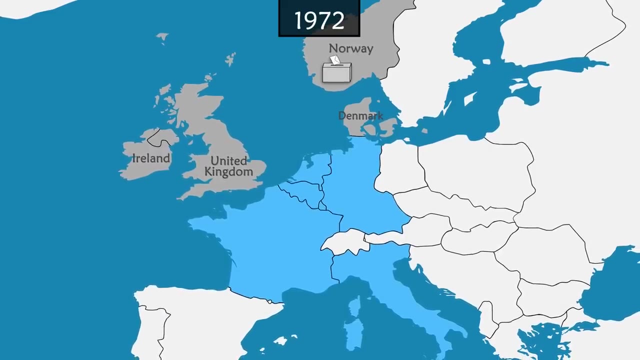 time. With the removal of tariffs for industrial and agricultural products and the free movement of workers, the economic situation improves rapidly, Prompting a new wave of membership applications. This time, negotiations go well, But in Norway, the population opposes the country's accession in a referendum. 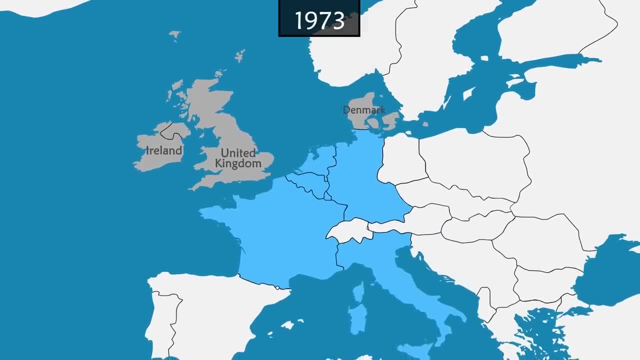 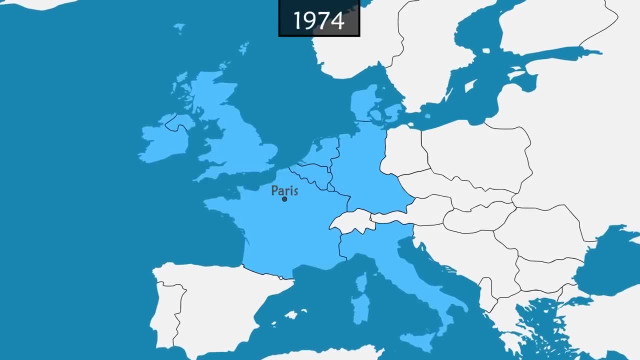 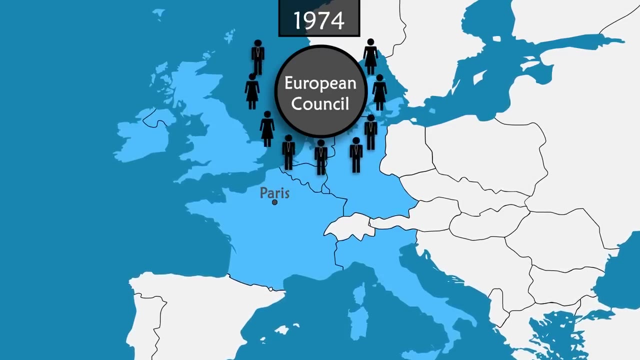 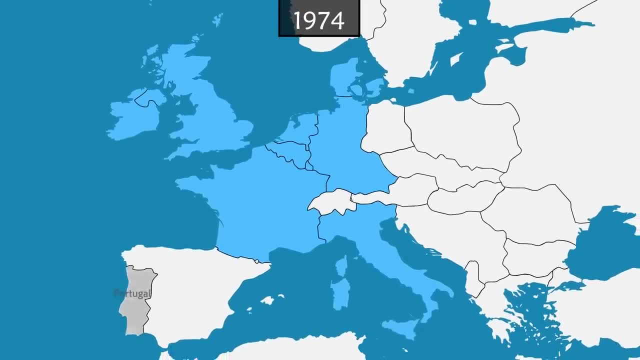 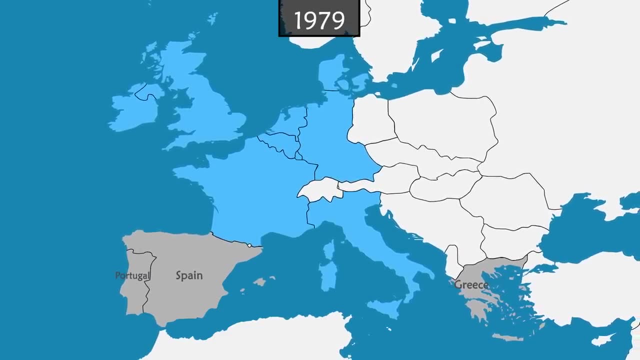 Both Thomeli and Riode find the broad guidelines of the Community South of the continent. after the end of dictatorships in Portugal, Greece and Spain, the three countries request membership of the Community In 1979, for the first time, members of the European Parliament are elected by universal 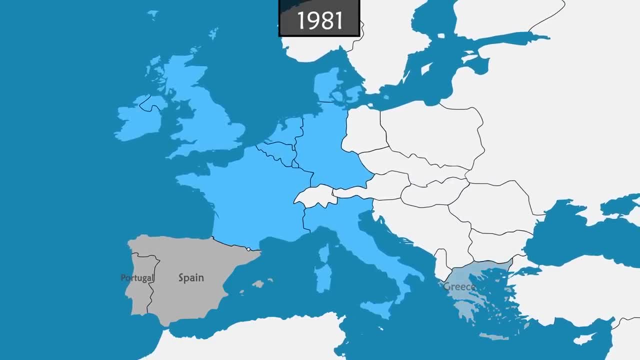 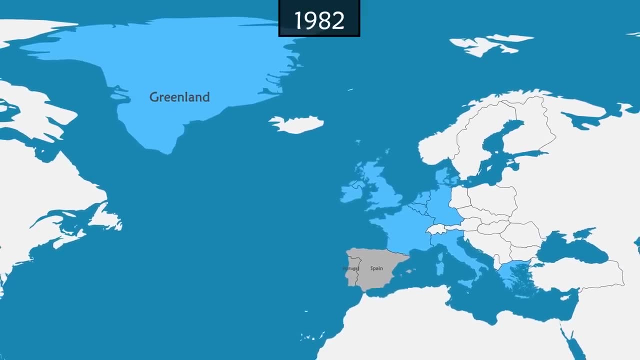 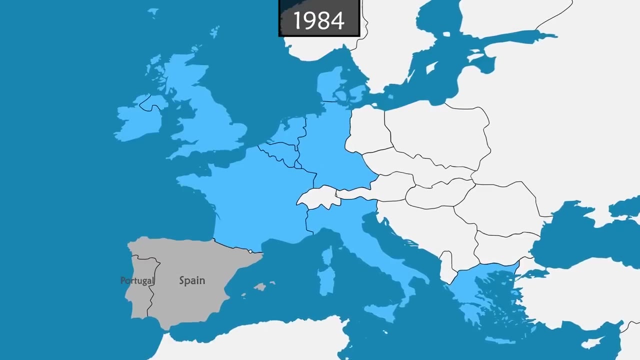 suffrage In 1981, Greece join the Community, while the following year Greenland, which receives more autonomy from Denmark, chooses to leave the Community. after a referendum In 1984, the United Kingdom under Margaret Thatcher says it does not benefit enough. 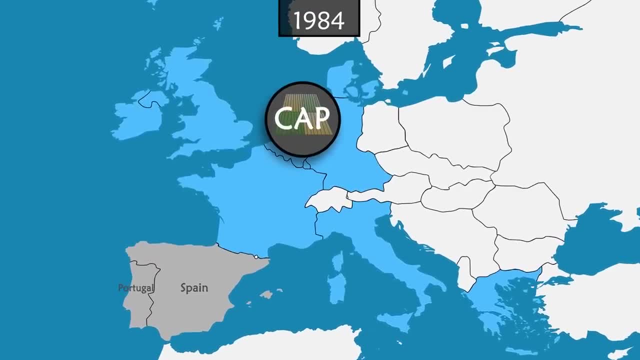 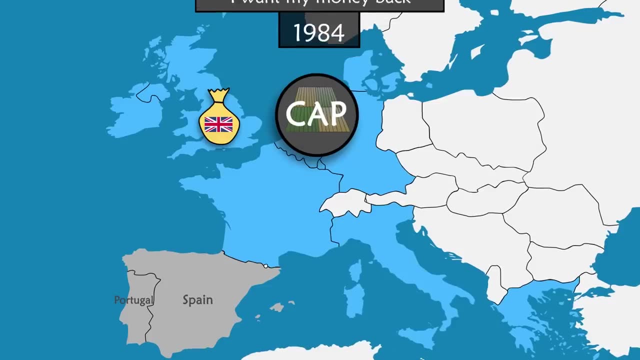 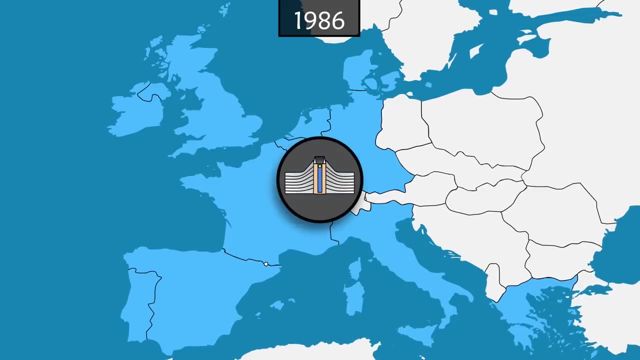 from the Common Agricultural Policy, which then represented 80% of EU spending. The country negotiates to obtain a reduction in its contribution to the community's budget. In 1986, Spain and Portugal join the community. Twelve member states and the European Commission give a boost to the internal market by signing. 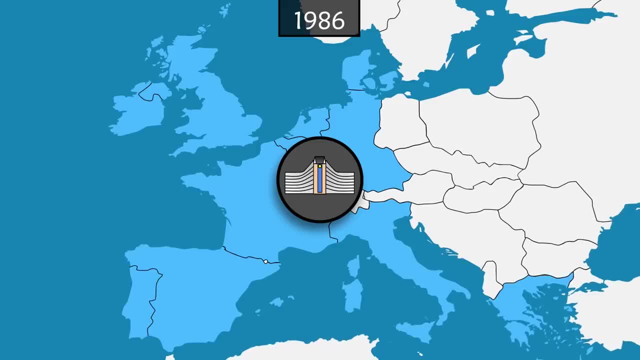 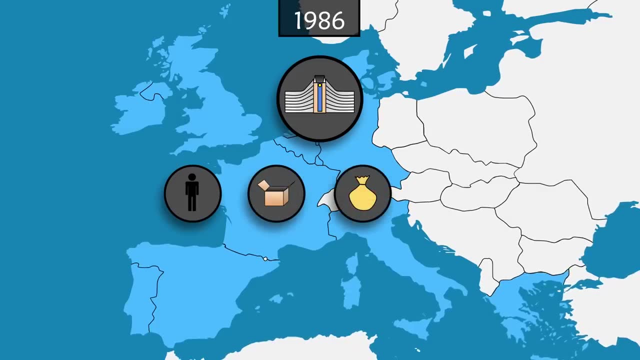 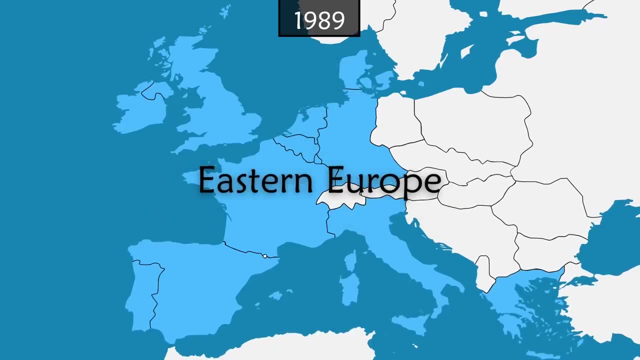 the Single European Act. In addition to eliminating custom fees, the goal is to remove all obstacles to the free movement of people, goods, capital and services. It is the single market project to be completed by 1993.. After the fall of the Berlin Wall, Germany is reunified. 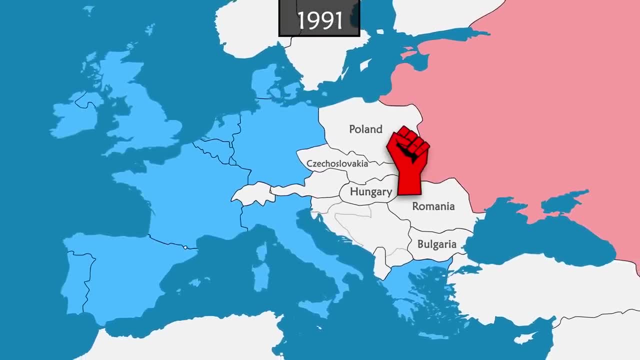 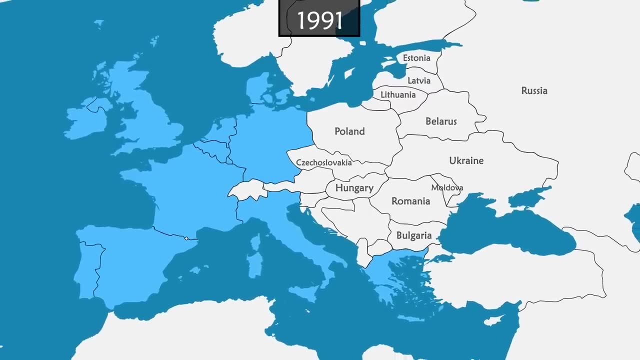 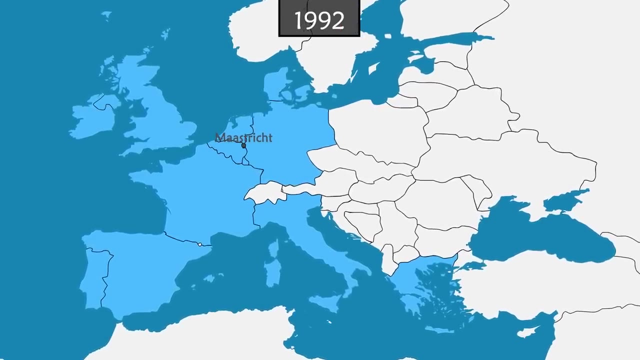 In the East. the USSR can no longer contain revolts and collapses, opening up new horizons for the community, which establishes contacts with the countries of Eastern Europe. On 7 February 1992, European heads of state sign the Maastricht Treaty. 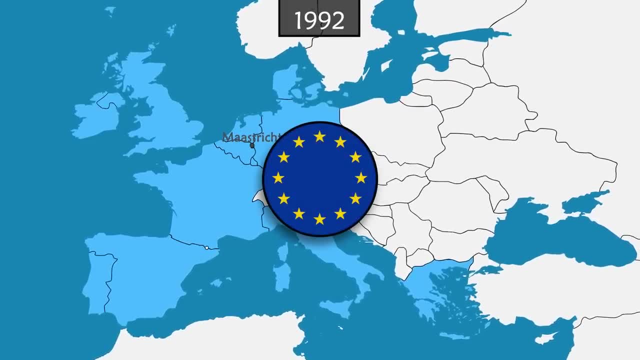 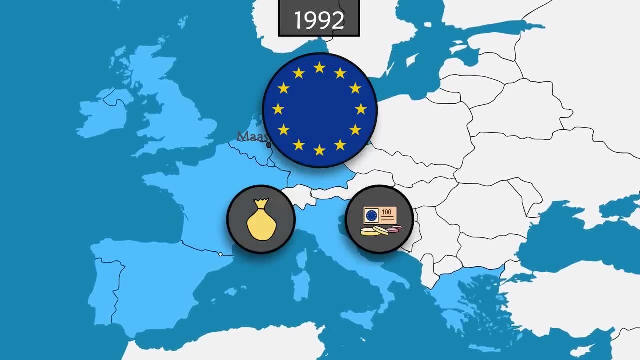 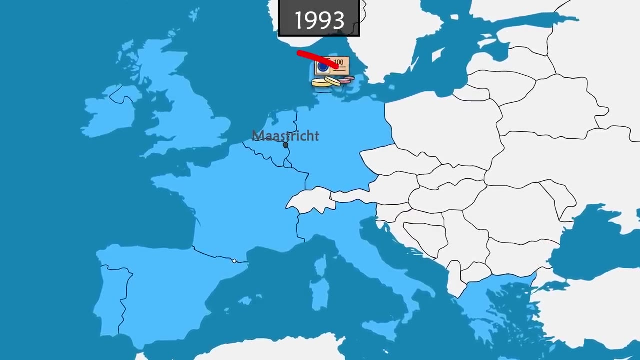 The European Union is created and gets new powers. The treaty envisages an economic union and the future creation of a common European currency. All countries ratify the treaty, including Denmark, where two referendums and negotiations to be exempted from the common currency are required. 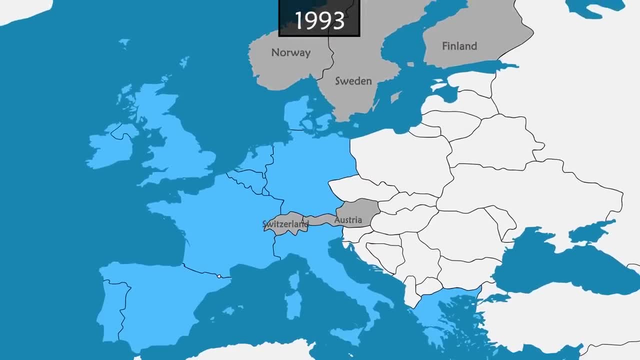 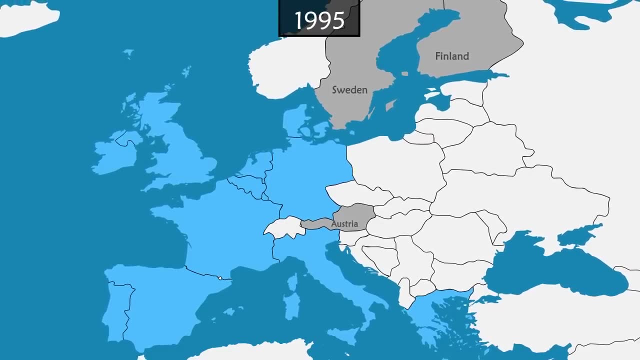 A new European Union is created. A new wave of countries request membership to the Union, But Switzerland and then Norway oppose potential candidacy via referendums. On the other hand, in Austria, Sweden and Finland negotiations succeed and in 1995,. 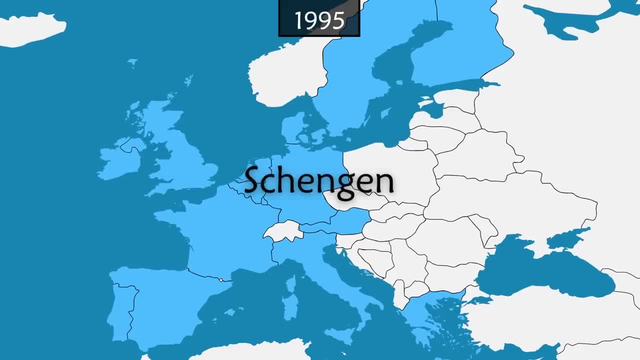 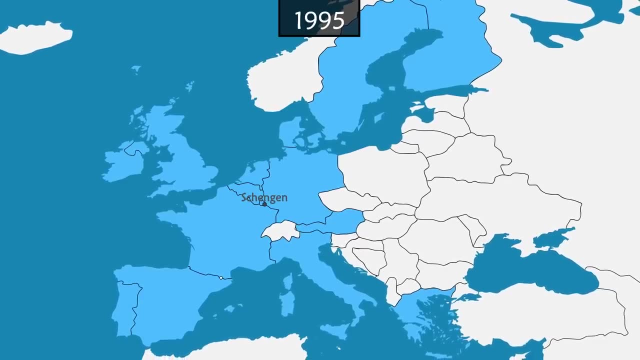 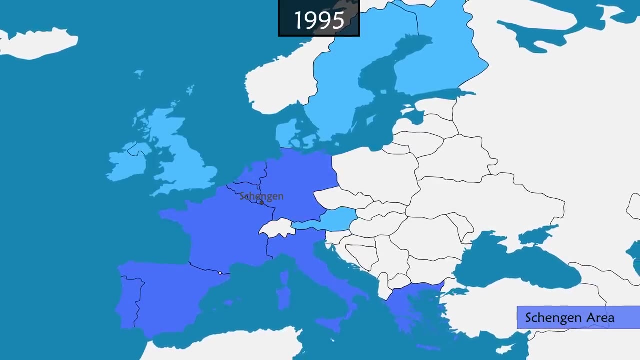 the EU grows to 15 members. Signed in Schengen-Luxembourg in 1985, the Schengen Agreement is gradually introduced from 1995.. Its objective is to abolish border controls and therefore have total freedom of movement within the European Union. 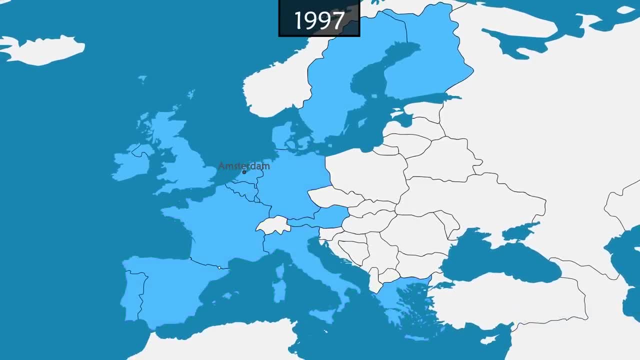 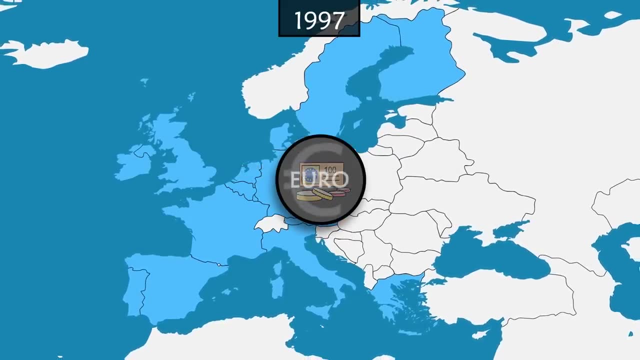 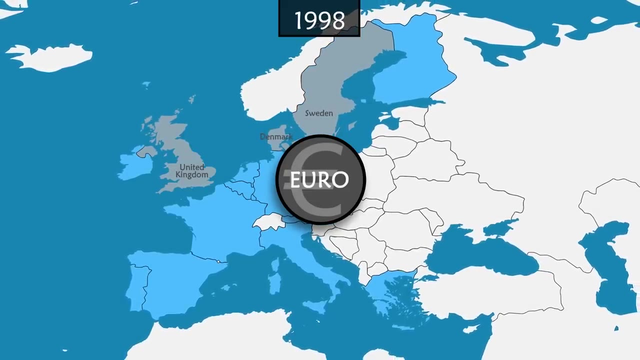 The agreement is incorporated into the European Union through the Treaty of Amsterdam. In addition, the common currency project advances, which would be called the Euro. However, the United Kingdom, Sweden and Denmark do not want it. The remaining member countries set up the European Central Bank. 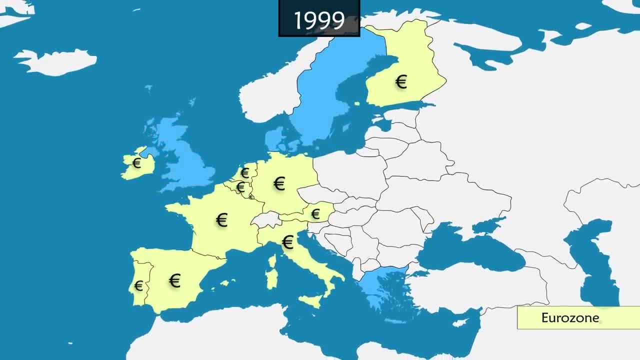 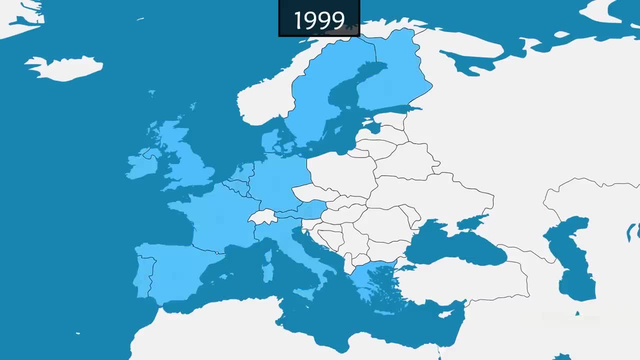 The Euro was the first European central bank. The Euro was the first European central bank. The Euro was officially launched on the market in 1999, although the currency would be put into circulation only from 1 January 2002.. As negotiations take place to enlarge, the Union heads of state meet in Nice to try 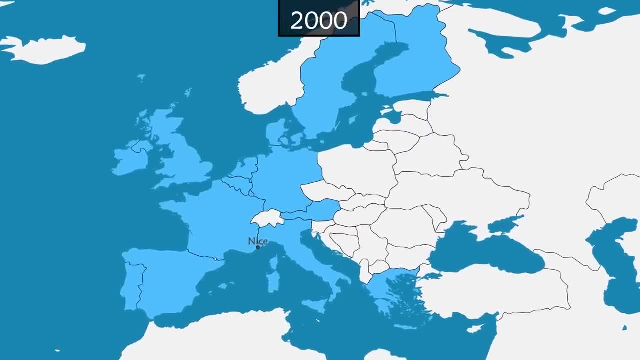 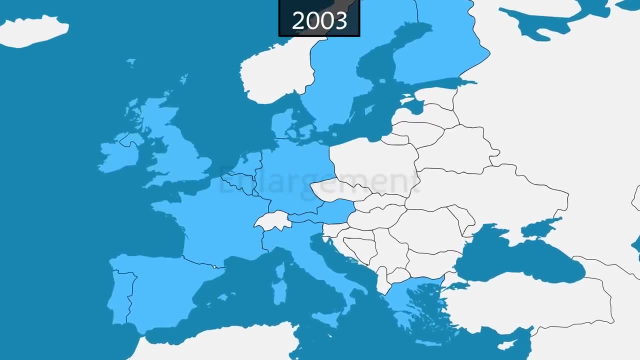 and improve the structure of the Union. The outcome of the Treaty of Nice is considered mixed. Two referendums are needed in Ireland for it to come into force, The first of May 2000.. The first of May 2000.. 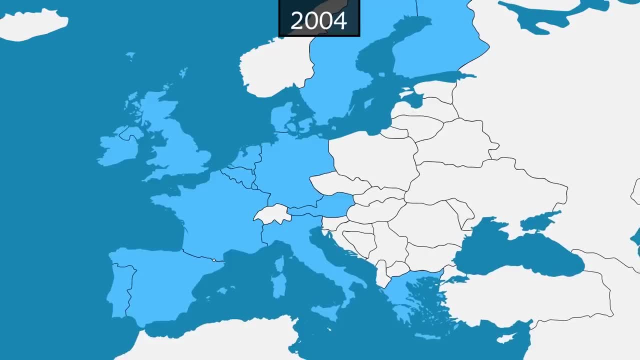 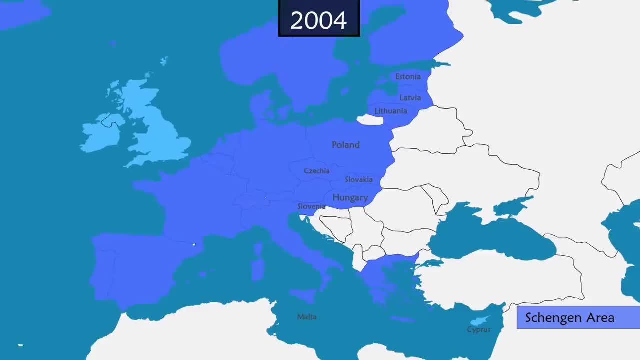 The first of May 2000.. The first of May long ago, in 2004,. ten new countries are included in the European Union. All new member join the Schengen area, with the exception of Cyprus, as part of the island is controlled by the Turkish army since 1974.. 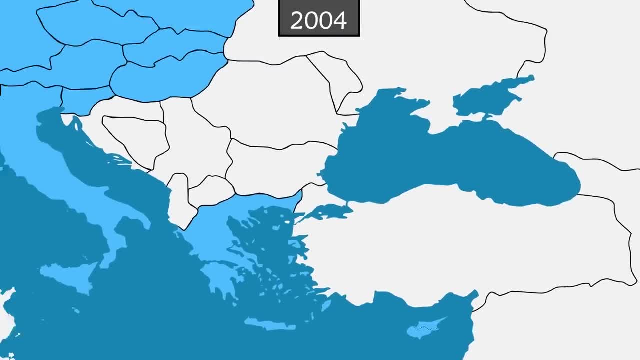 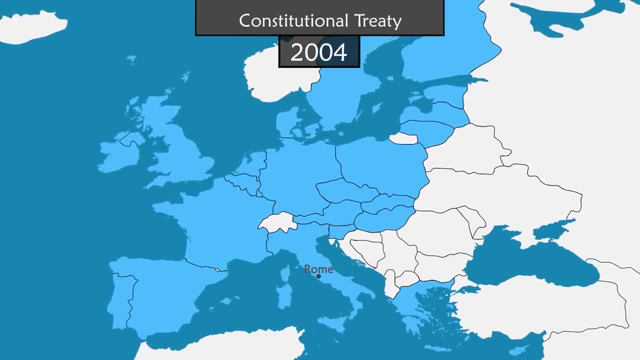 After the half failure of the Treaty of Nice, 25 heads of state meet in Rome again to try to streamline the functioning of the European Union. This time they aim to create a constitutional treaty which would replace all existing treaties with a single text. 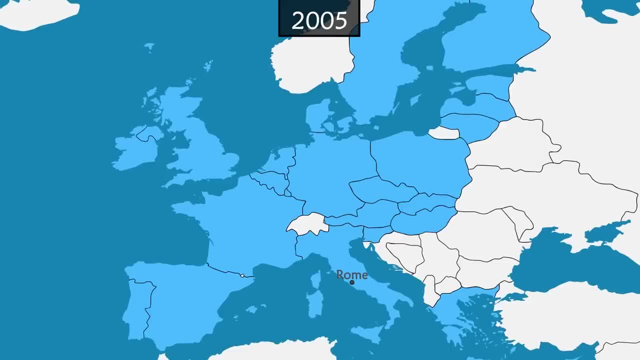 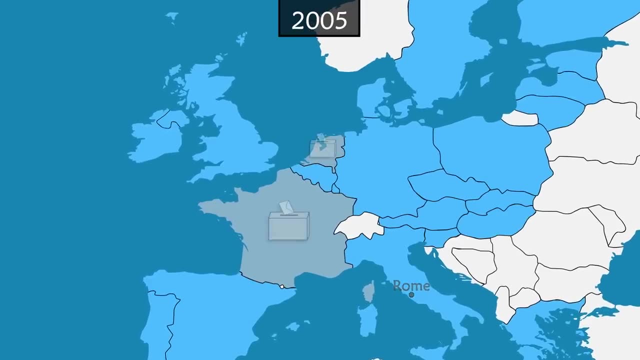 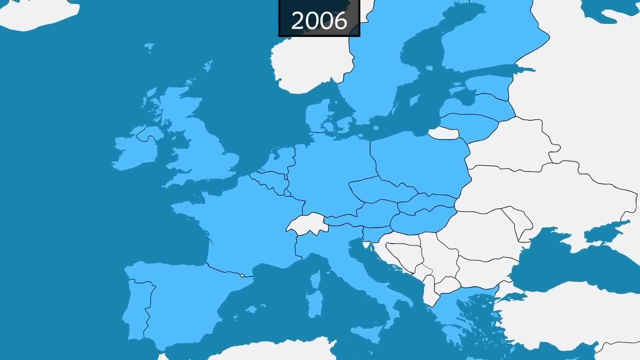 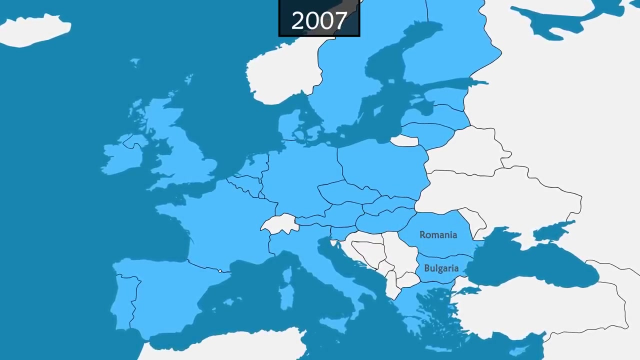 fixed. This sparks heated debate across Europe. Fearing an overly powerful European Union at the expense of national sovereignty, the French and Dutch populations oppose the treaty via referendums. This triggers a period of reflection and in-depth consultation within member states. On January 1, 2007,, Romania and Bulgaria joined the European Union. 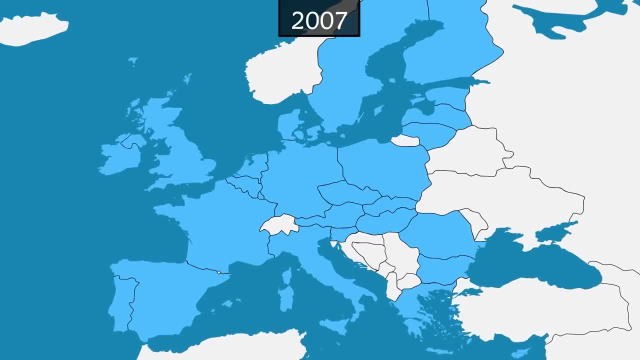 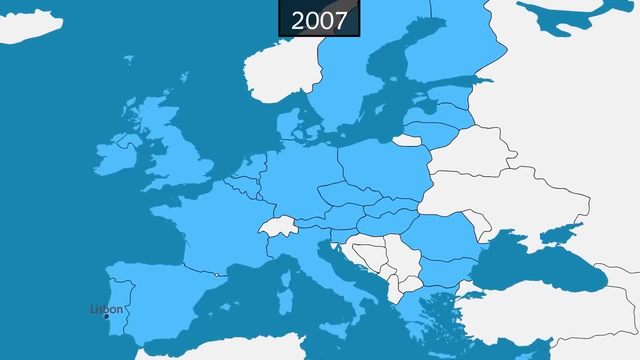 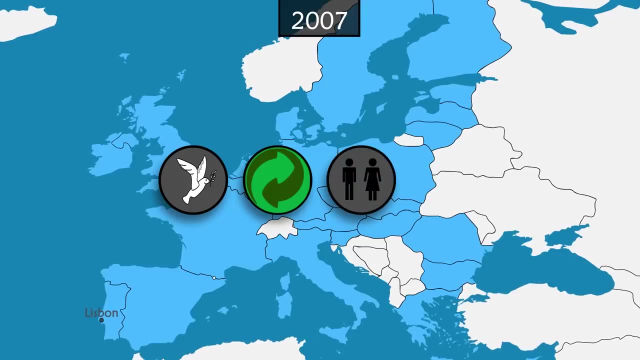 The same year, 27 heads of state signed the Treaty of Lisbon, which aims to strengthen and improve the functioning of the EU after enlargement. Notably, it is agreed that the EU's role is to promote peace, support sustainable development, fight against social exclusion and discrimination, and safeguard cultural heritage. 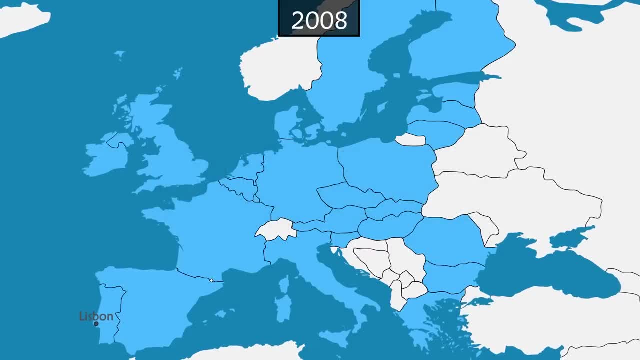 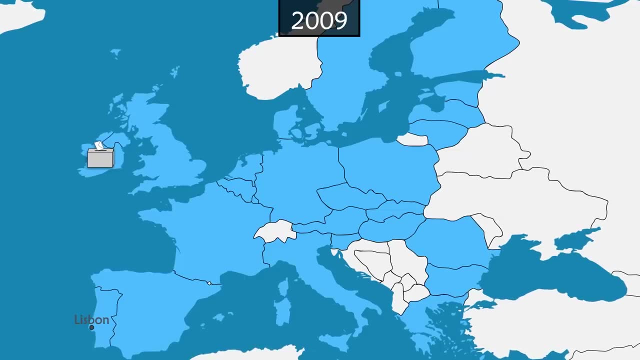 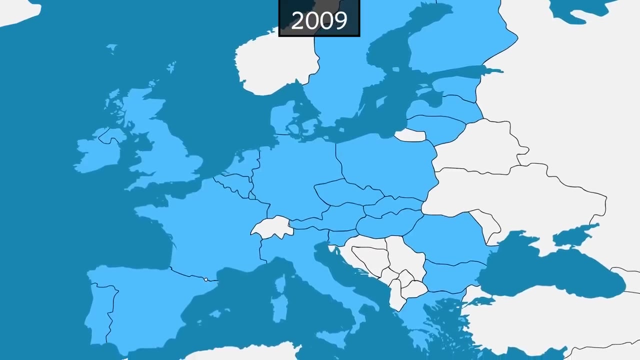 The treaty is ratified by all states but Ireland, which holds a referendum and rejects it. Yet again, more negotiations and a second referendum would be needed in Ireland for it to take effect. The global economic and financial crisis has repercussions on the Eurozone, which enters. 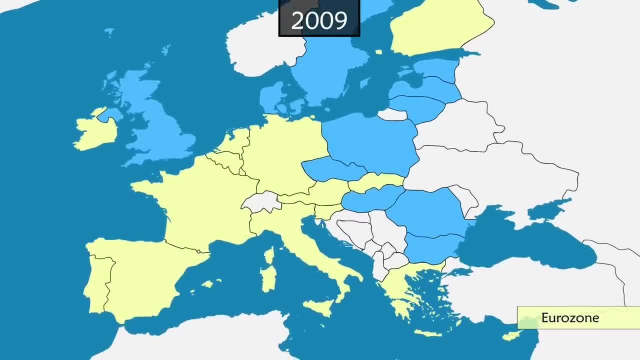 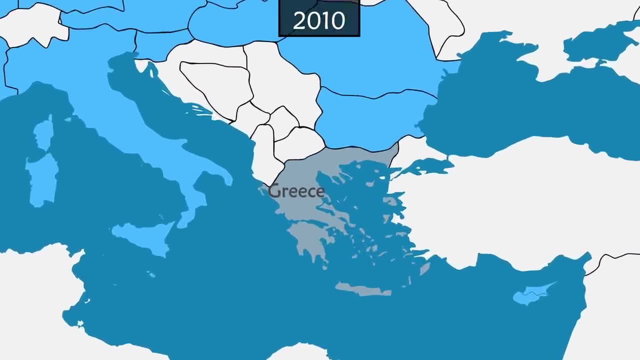 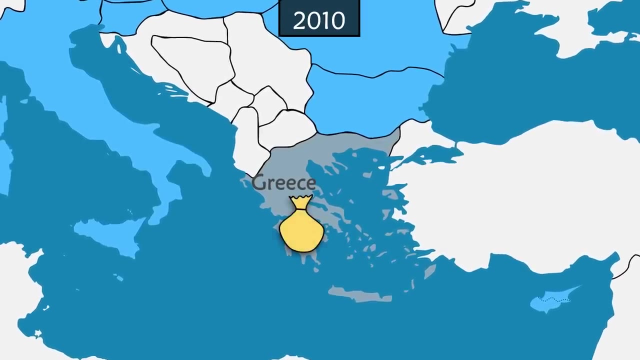 a recession After the rout of major European banks. many countries find themselves in difficulty, In particular Greece, part of whose public debt has been kept hidden with the help of consultants from the Goldman Sachs Bank. The country is forced to ask for financial aid from the Eurozone and the IMF in exchange. 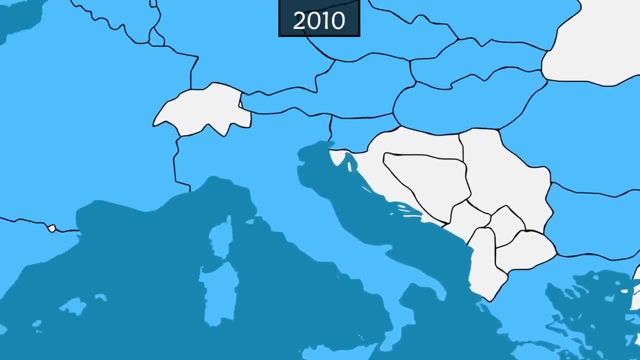 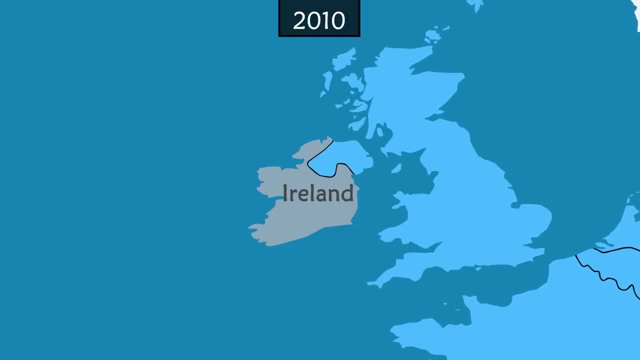 for which it must implement austerity measures. Ireland, coming to the aid of its banks, also sees its public debt explode, But the country does not want to ask for aid from the Eurozone, fearing it may, in return, be forced to raise its low corporate tax rates. 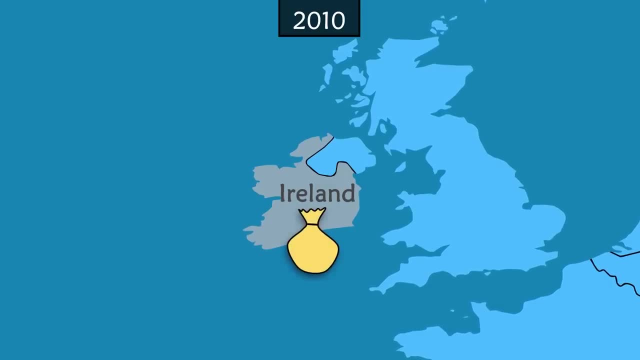 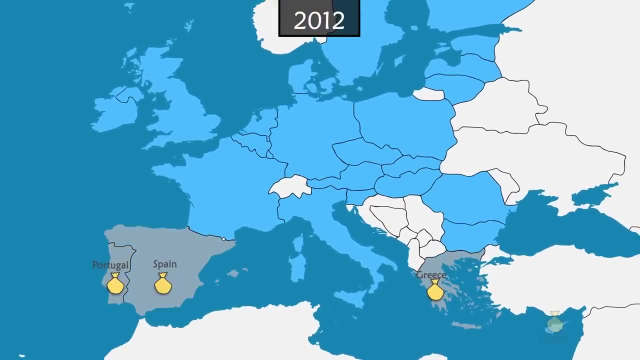 The country finally receives aid all the same, in exchange for which it must adopt a strict plan. Subsequently, Portugal, Greece, a second time Spain and then Cyprus obtains financial aid from the Eurozone, While almost everywhere on the continent, the Eurozone is the only country to receive. 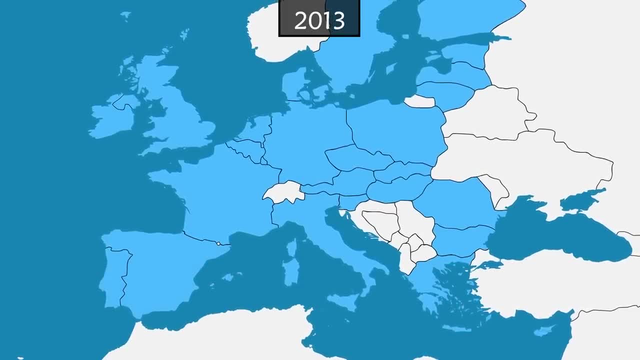 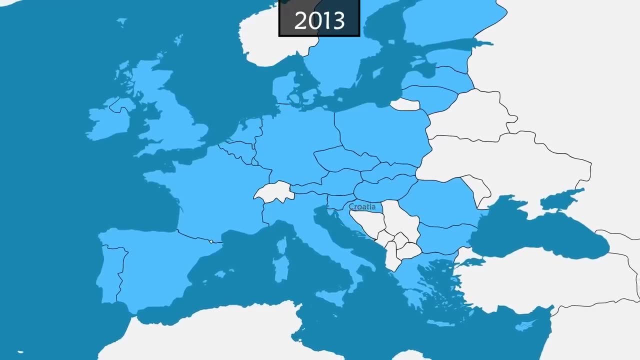 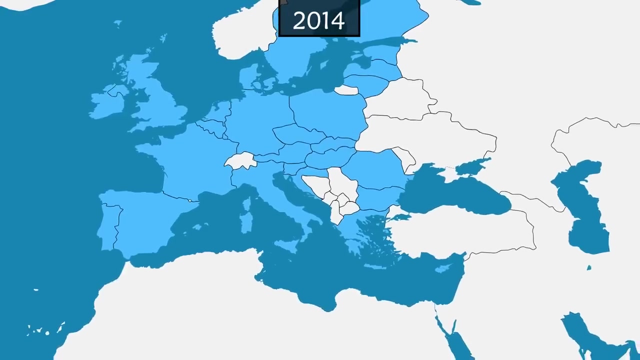 financial aid In 2013,. Croatia joins the European Union. At the borders of the continent, the so-called Arab Spring creates instability in many countries. The civil war in Syria, a second civil war in Libya and in Iraq, and other events such 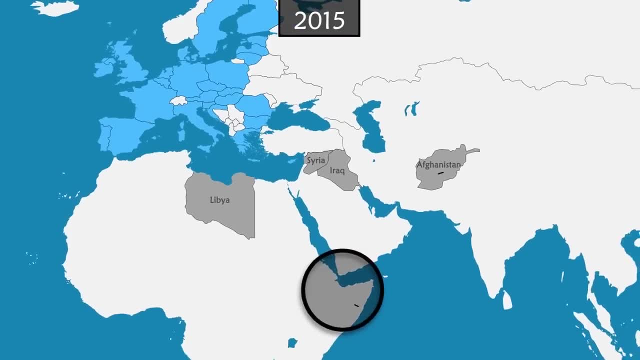 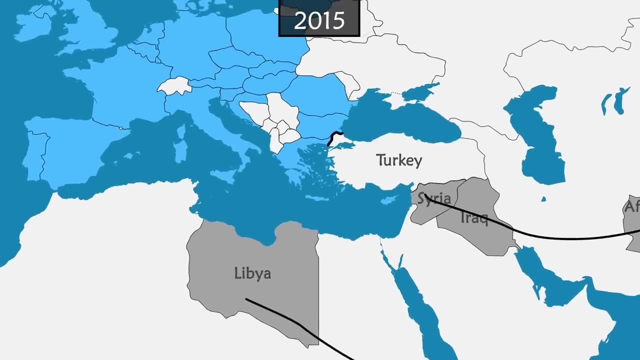 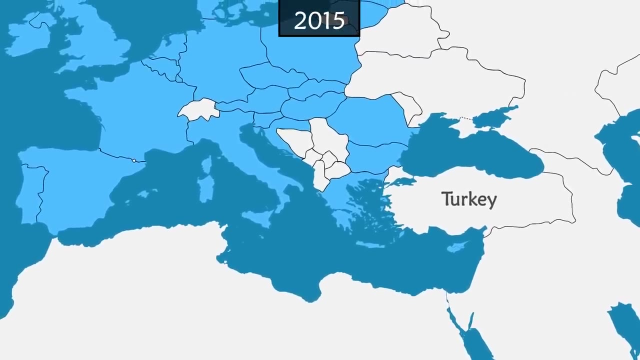 as the war in Afghanistan and violence in the Horn of Africa push many people to migrate to Europe. Despite the construction of walls at the Turkish border in 2015,, over a million migrants enter the Schengen area. Europe tries to slow the flow of migration. 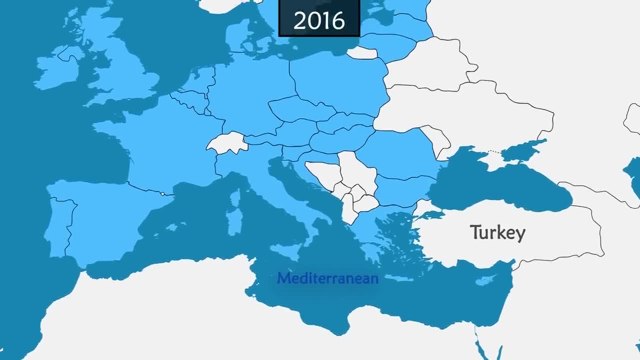 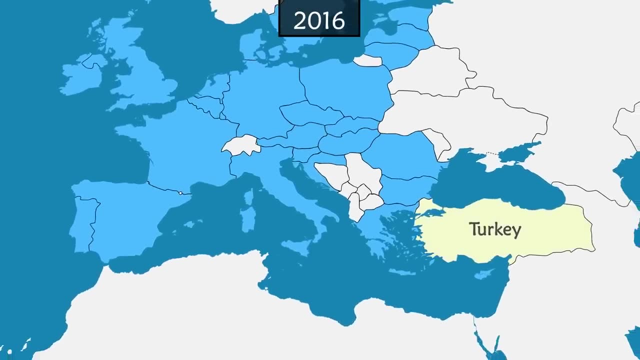 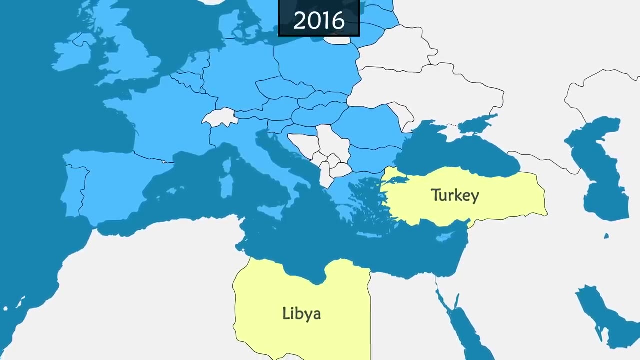 Security patrols are reinforced on the Mediterranean Sea, while certain countries temporarily reintroduce controls at their borders. In addition, the European Union signs agreements with Turkey and then with Libya, where the political situation is very unstable, so that they control and block the so-called Arab Spring. 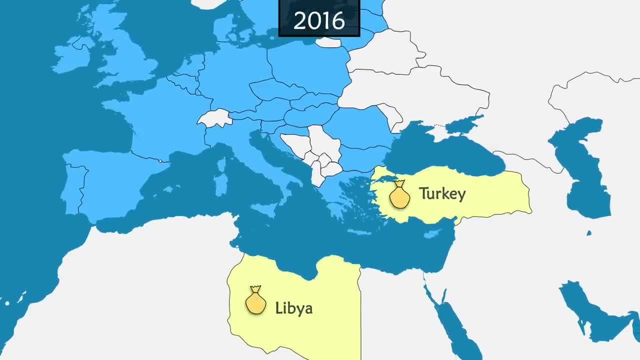 In 2016,. the European Union has found debt to the European Union, but has not yet reached the minimum wage. The European Union has called for a permanent break from the sovereign security policy. Migrant processing centres have been expanded in the EU in order to reduce the debt of. 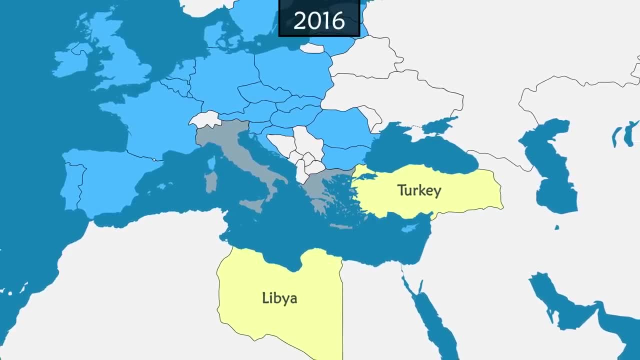 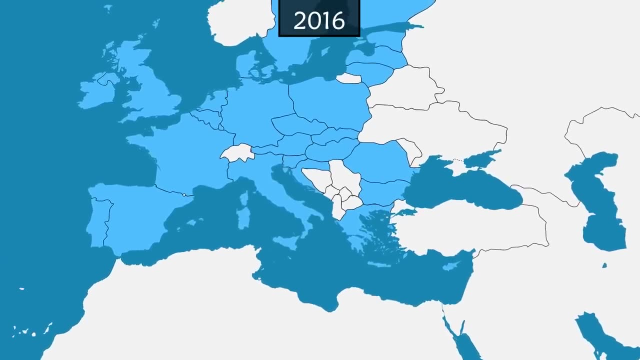 migrants, and the EU is now building new training and training centres in Greece and Italy to help migrants with international bases in the EU, Migrant processing centres are funded mainly in Italy and Greece, where migrants find themselves awaiting regularization in overcrowded conditions. The migration crisis divides European countries and fuels the rise of nationalist and Euro-sceptic. 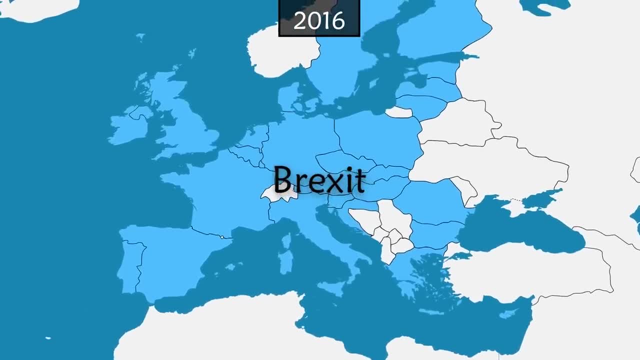 parties. The EU has also provided Europe with funds: % In June 2016, the United Kingdom, through a referendum, votes in favour of vowing to stop the EU from becoming a nuclear power- A reverb, as the European Union says failed to do. 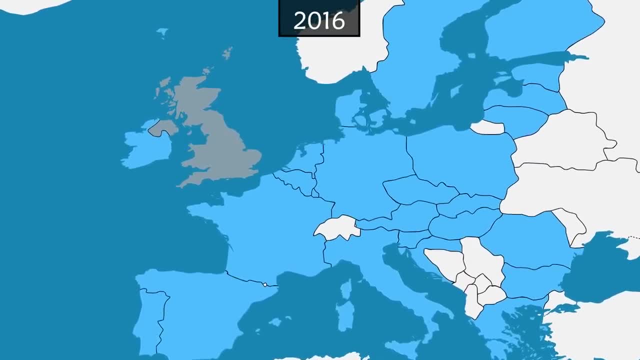 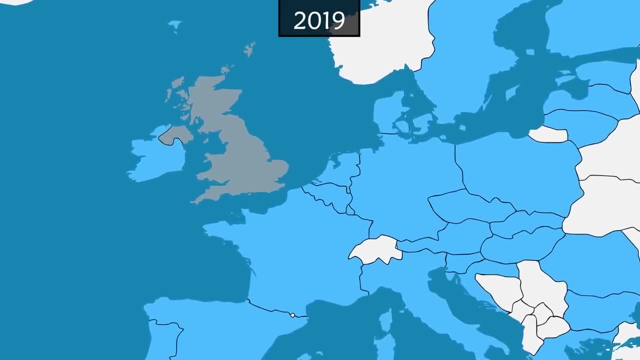 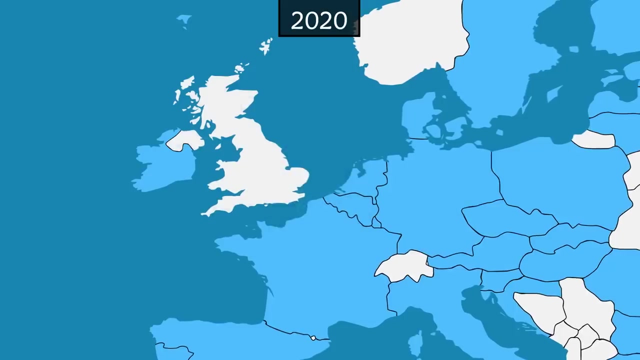 leaving the European Union. The country then enters long and difficult negotiations with the European Union to define the conditions of their withdrawal. After numerous failures, an agreement for Brexit is finally reached and the United Kingdom exits the EU on January 31, 2020.. 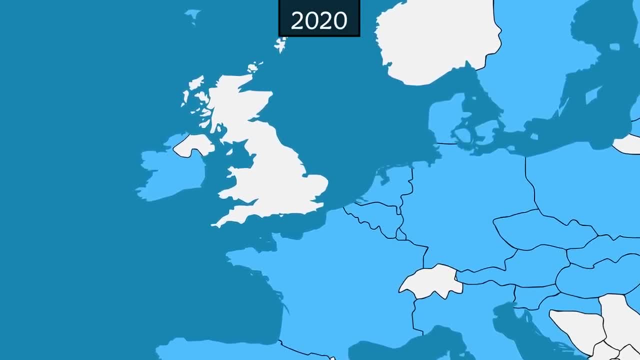 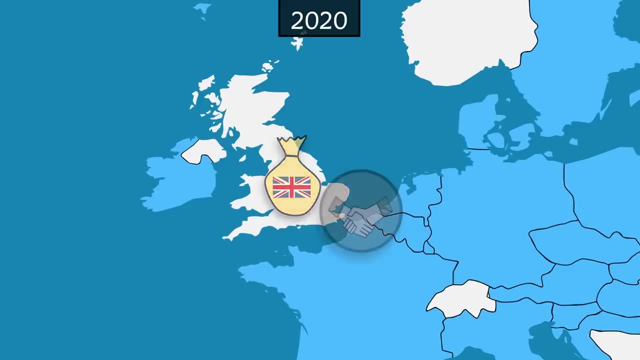 While the UK no longer has any decision-making power in the bloc, it continues to contribute to the European budget and receive funding, at least until the end of the year. By this deadline, it is meant to negotiate future agreements with the EU, in particular.